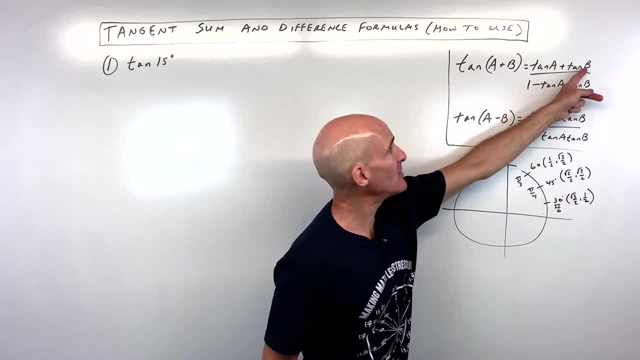 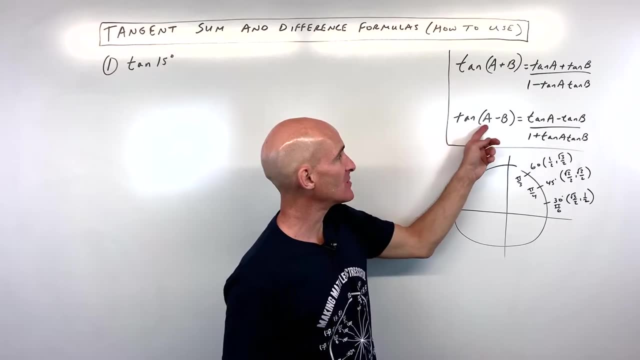 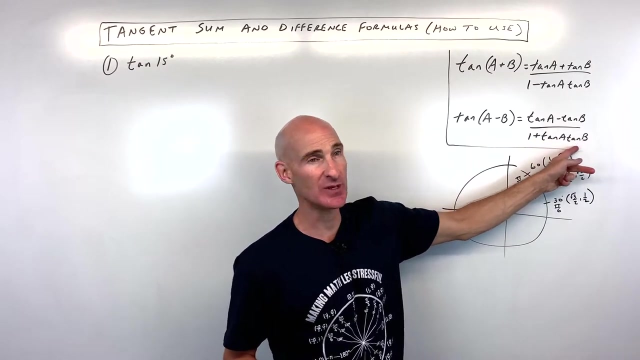 angles. notice how it's tangent of a plus tangent of b and the denominator it's the opposite: one minus tangent of a times tangent of b. Over here we're subtracting tangent of a minus b, See tangent of a minus tangent of b. The denominator is the opposite: one plus tangent of a times tangent of b. 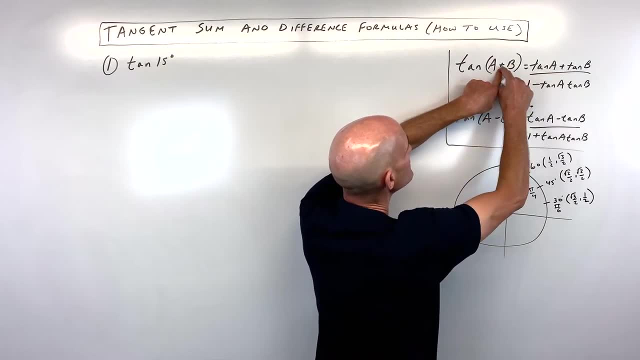 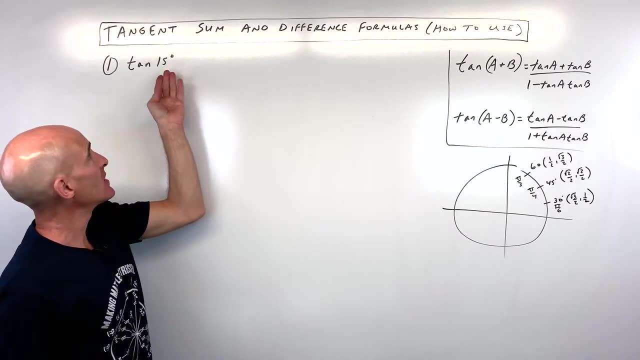 So sometimes they'll group them together, They'll say like this is plus, plus, if this is minus, they'll put like a little minus there. So it's kind of a you know, condense it a little bit less for you to memorize. But the question we want to ask ourselves is: you know, we're not familiar with. 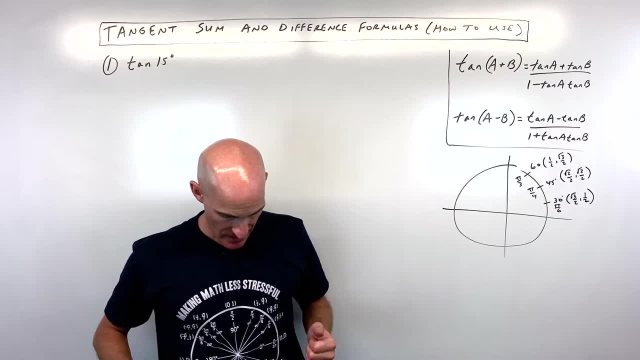 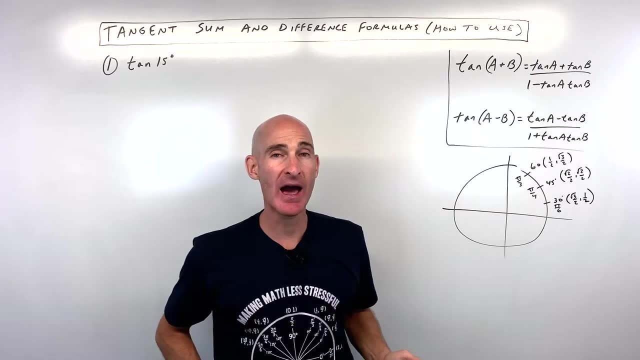 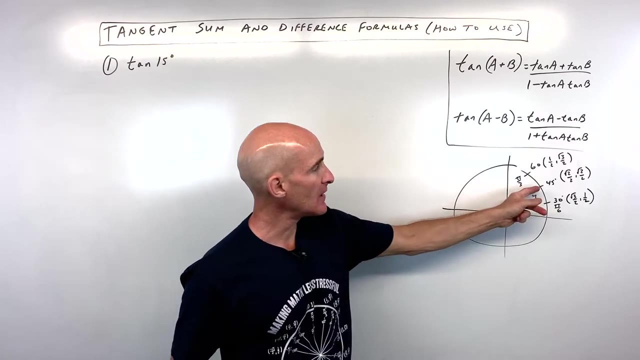 the unit circle- I wore my unit circle t-shirt here today- is there's not a 15 degrees on this unit circle. So we have to figure out what two angles can we add or subtract to get 15 degrees. So there's more than one option. but why don't we just keep it simple and we'll say: 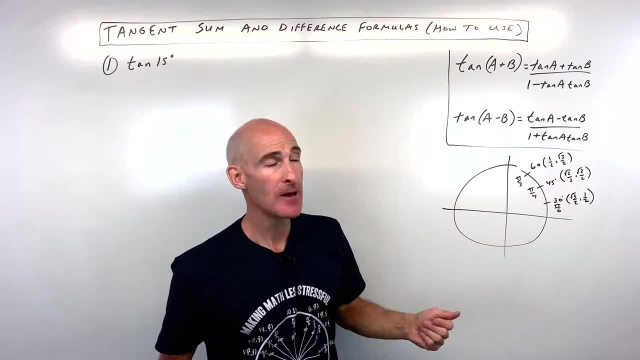 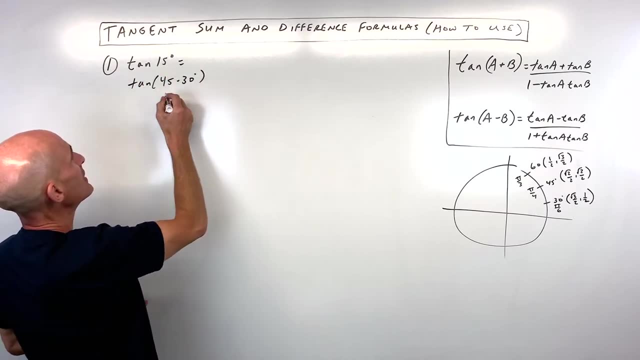 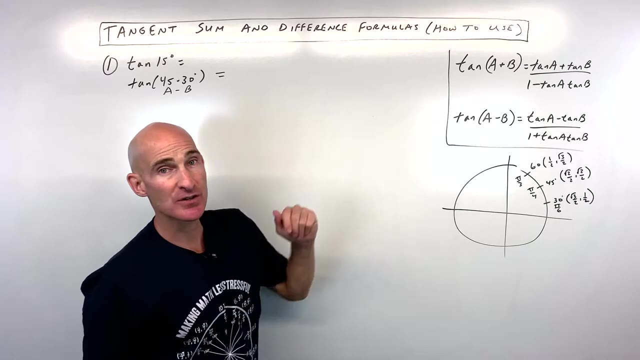 45 minus 30. That gives us 15.. So let's write that down. So we're just going to say this is the same as tangent of 45 minus 30. So this is our a- 45. And b is our 30. Let's go ahead and expand that out using our tangent difference formula. So we 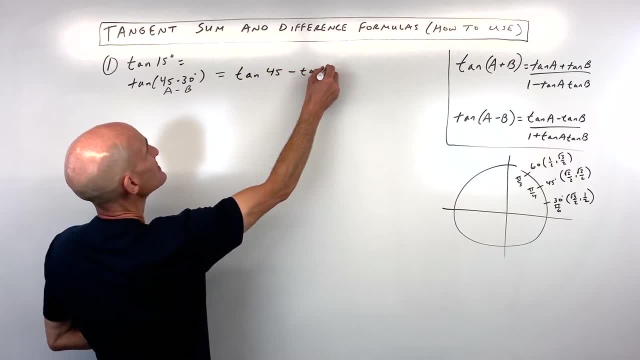 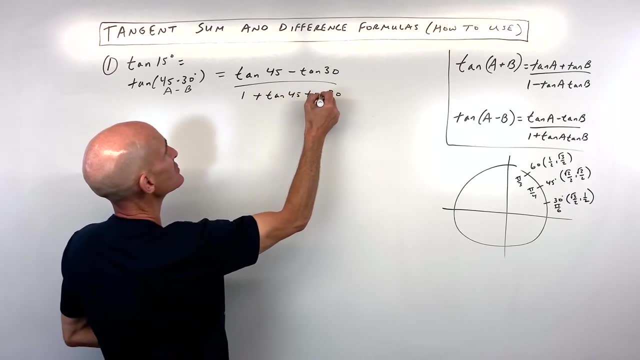 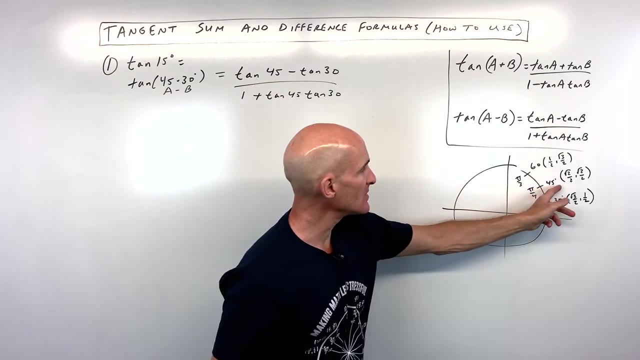 have tangent of 45 minus tangent of 30 over 1, plus tangent of 45 times tangent of 30. Now, with the unit circle, tangent is the y coordinate over the x coordinate. So we go to 45 degrees: y divided by x, square root of 2 over 2 divided by square root of 2 over 2.. That's 1 because 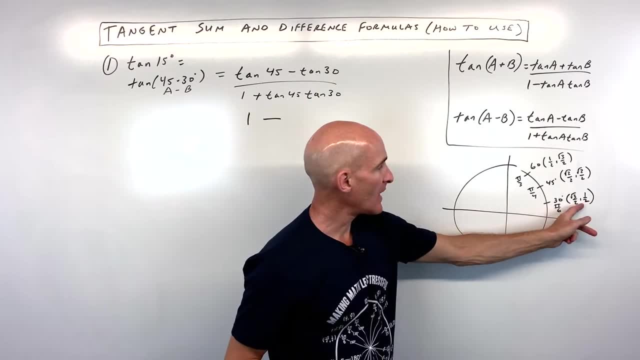 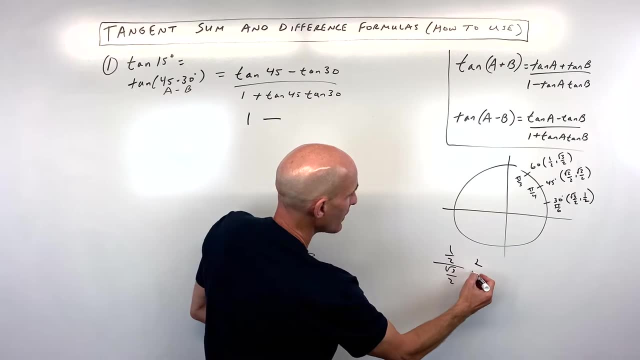 1. Tangent of 30 is 1 half divided by square root, 3 over 2.. So let's go ahead and do the work over here: 1 half divided by square root, 3 over 2.. If we multiply the numerator and denominator by 2, 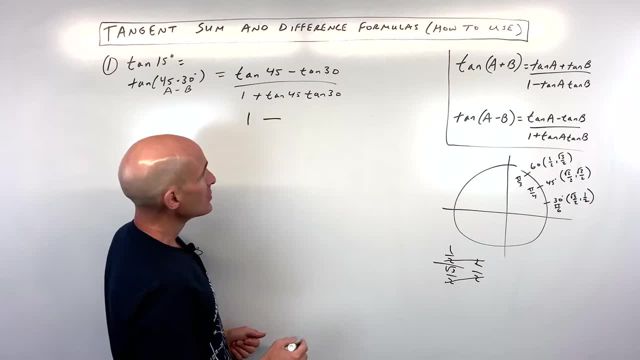 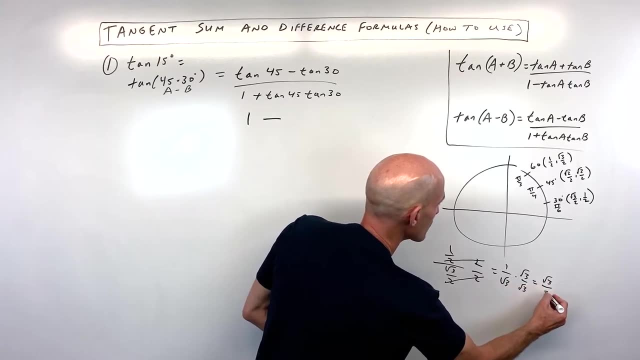 see how you get 1 over square root of 3.. So you can rationalize that to: let's multiply the numerator and denominator by square root of 3.. So that comes out to square root of 3 over 3.. So root 3 over 3. 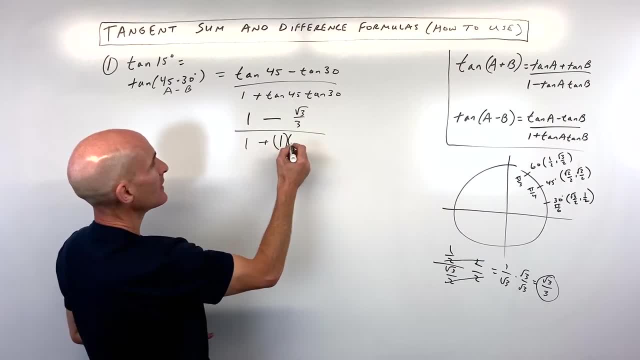 1 plus the tangent of 45, which we said was 1.. And the tangent of 30, we said was square root of 3 over 3.. Okay, so let's simplify a little bit more now. So we've got 1 minus square root of 3 over 3.. And 1 times anything is itself, So square root of 3 over 3.. 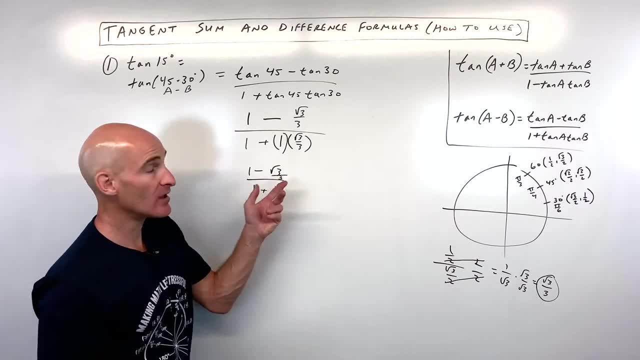 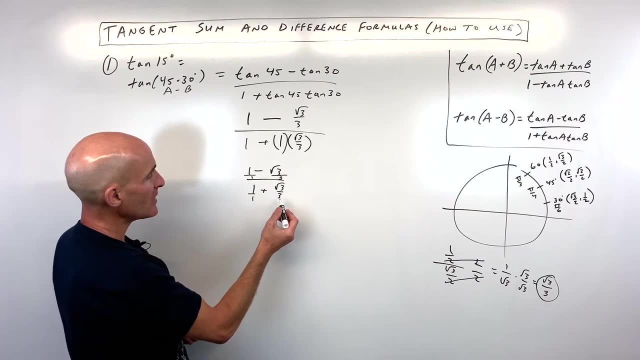 Now this is what we call a complex fraction, because we have fractions within a larger fraction. What I'm going to do is I'm going to clear the denominators. 1 is like 1 over 1.. This is like square root of 3 over 3.. The common denominator is 3.. So if I multiply the numerator by 3 and I, 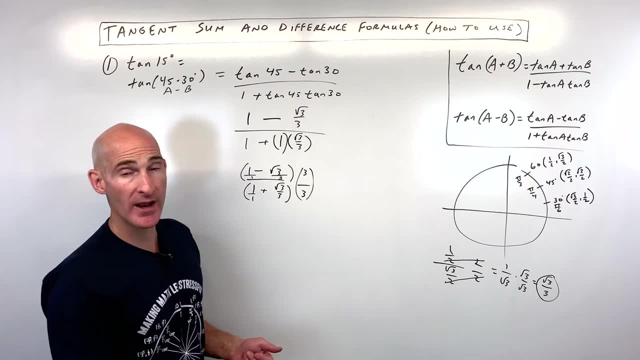 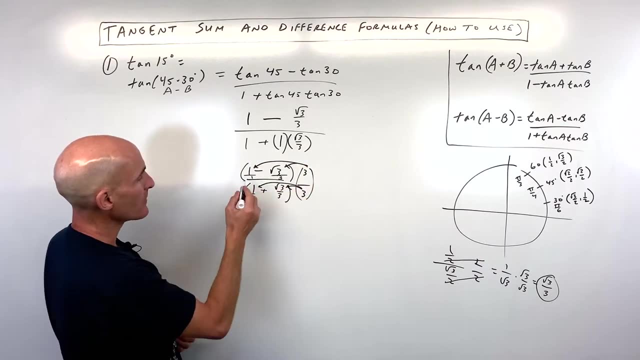 see: 3 divided by 3 is like 1.. So 1 times anything doesn't change the value. What it's going to do, though, is going to clear the denominators, So I'm distributing that 3 in there. So 1 times 3 is 3.. 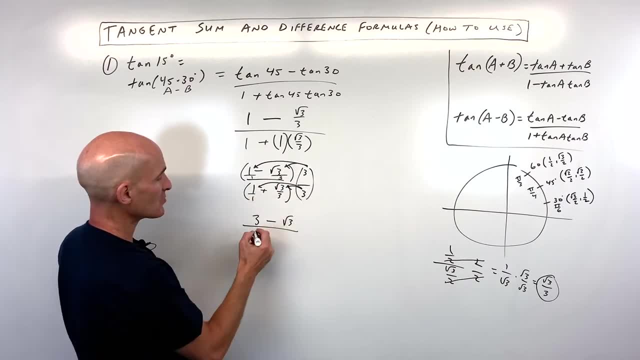 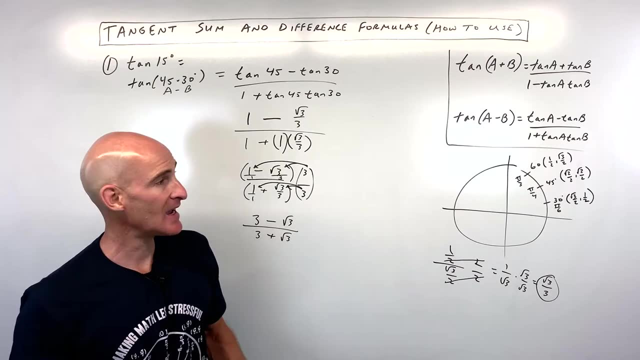 Here these 3's cancel. That's square root of 3.. 1 times 3 is 3.. Here these 3's cancel and we get square root of 3.. Now some teachers will let you leave it like this. They'll say: you got the basic. 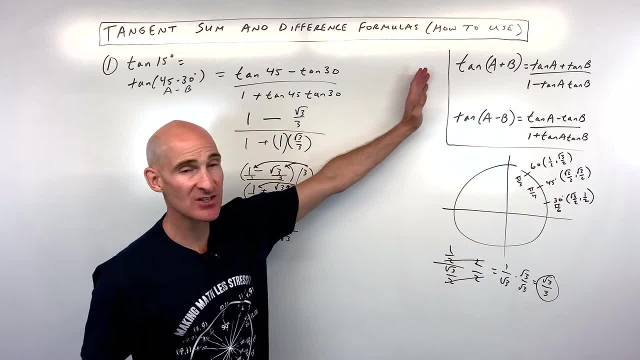 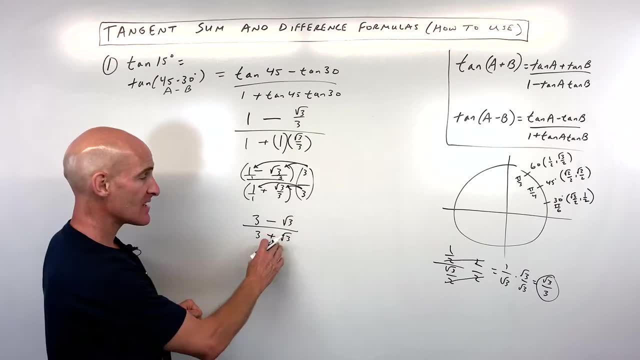 idea. You know how to work with the unit circle. You know your tangent sum and difference formulas Further, by rationalizing the denominator. But other teachers will say, well, it's not considered proper to have that square root in the denominator. So how do we get rid of that square root in the 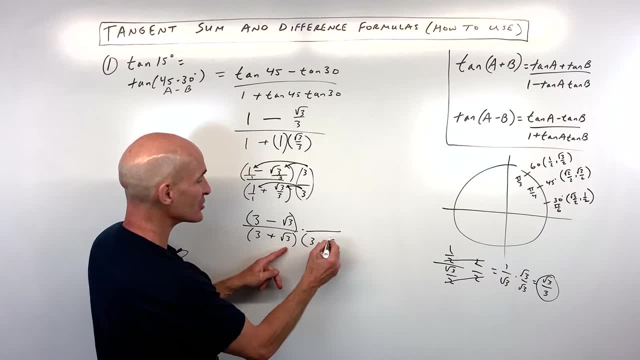 denominator, We multiply by the conjugate. So if this was 3 minus square root of 3, I'd multiply by 3 plus square root of 3.. Notice, I'm just changing that sign in between. Okay, the two terms. Whatever you do to the denominator, you want to do to the numerator, because it's like multiplying by 1.. 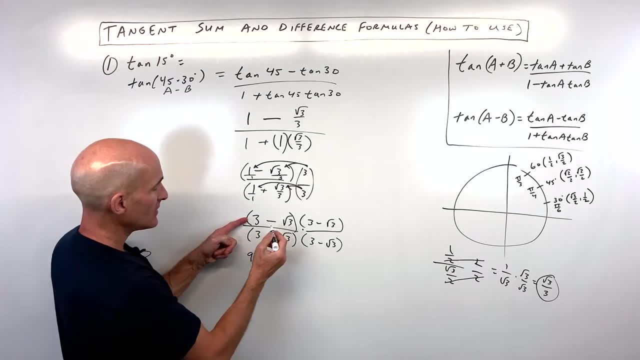 And now we're going to FOIL. So we have 3 times 3, which is 9.. 3 times negative root 3 is 9.. Negative 3 root: 3. Negative root 3 times 3 is another negative 3 root: 3. Negative root: 3 times. 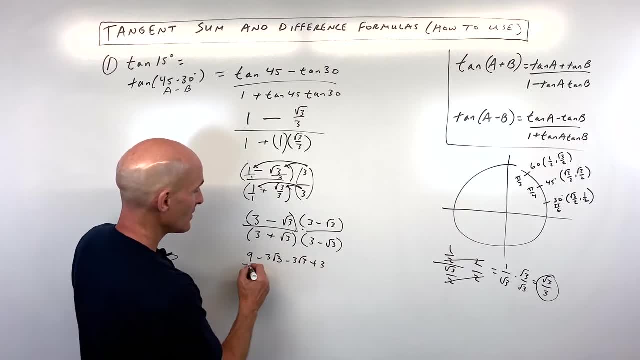 negative root. 3 is positive square root of 9, which is 3.. Okay, and then over here, 3 times, 3 is 9.. 3 times negative root 3 is negative root 3.. Basically, the outer and the inner are canceling. 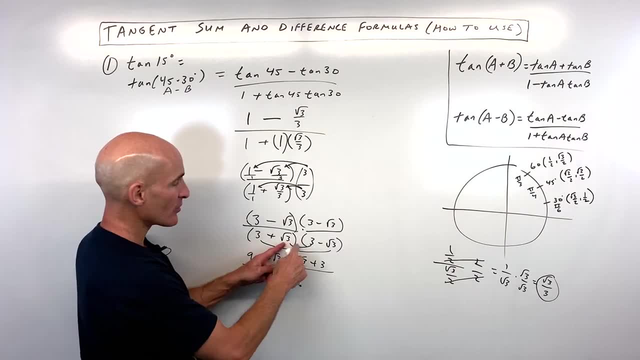 3 root 3 and negative 3 root 3, those cancel And then square root of 3 times negative, square root of 3, that comes out to negative 3, because that's square root of 9.. Square root of 9 is 3.. Positive: 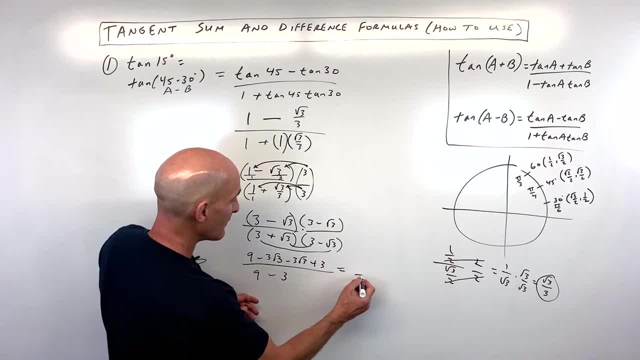 times a negative is a negative. But notice we got rid of the square root in the denominator. Okay, so that comes out to 6.. 9 plus 3 is 12. And this comes out to negative 6 root 3.. 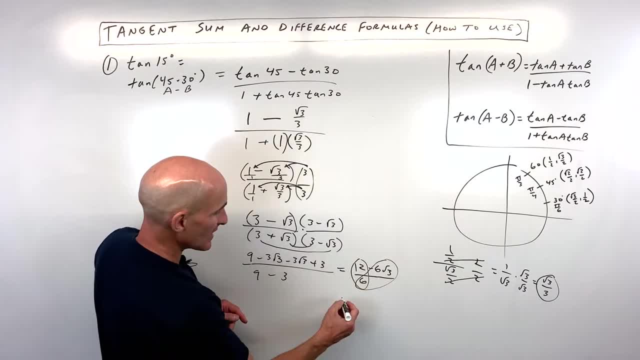 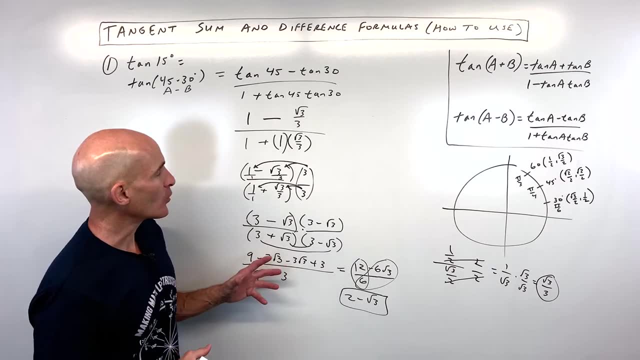 Now you can divide both of these terms by 6. And you can write this as 2 minus square root of 3. And that's about as far as we can simplify that one. So I know I went kind of quick on that, But. 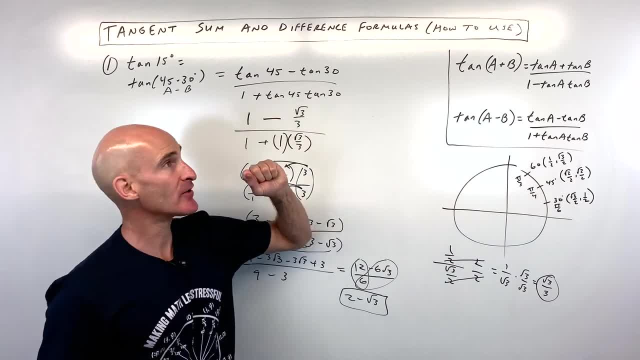 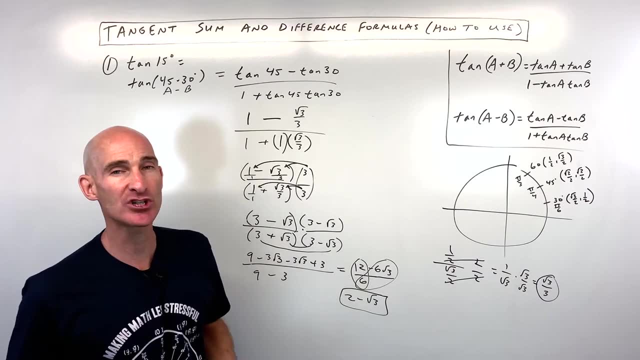 the key is to recognize what angles are going to add or subtract to 15. And then you substitute and just do the arithmetic. But let's look at another example, using radians. This can be a little bit more challenging. And I also want to say: if you want to get one of these t-shirts, 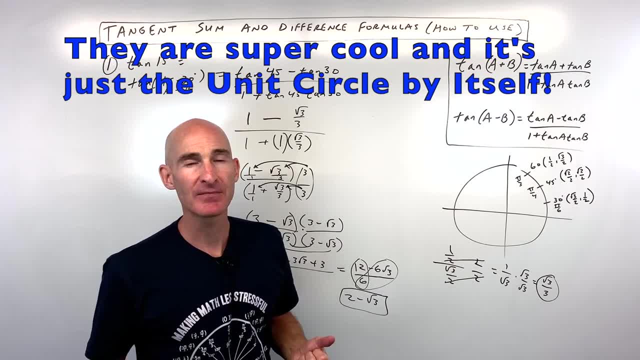 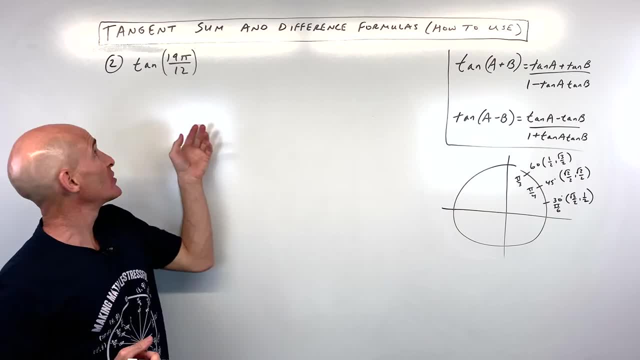 you can go to the store on my YouTube page or you can go to the description. I'll have a link for these t-shirts, So they're also on the merch shelf below the video. Okay, example number two: We're going to do the tangent of 19 pi over 12.. Now, if you're like me, you're probably like: 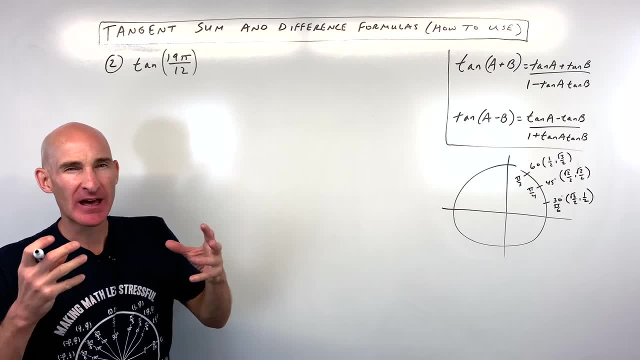 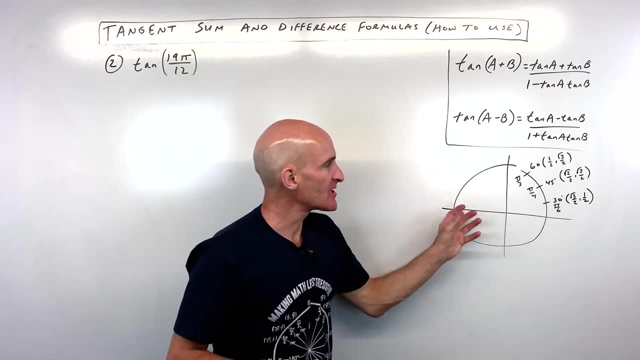 what angle is that right? And some people are really good, you know, about figuring it, kind of working backwards and saying, well, hmm, if I took like 5 pi over 4 plus, you know. But what you want to do is you want to make sure it's the sum. 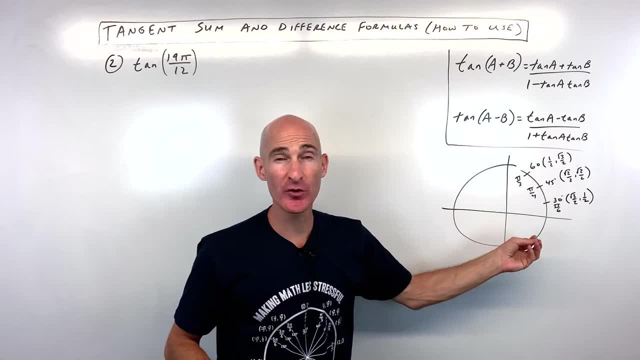 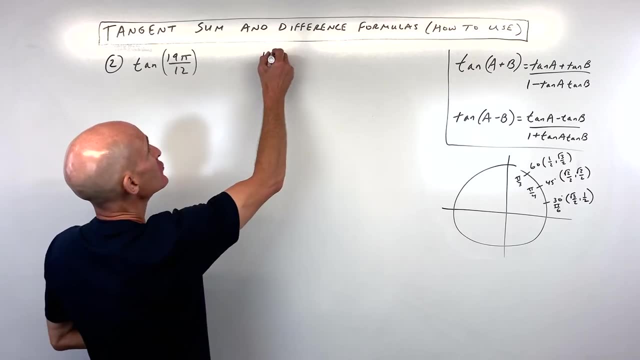 of two angles that you're familiar with, or the difference of two angles that you're familiar with on the unit circle, right. But what I like to do is I like to convert this to degrees first. So let's just go ahead and do that. So we have 19 pi over 12 times 180 degrees for every pi radians. That's. 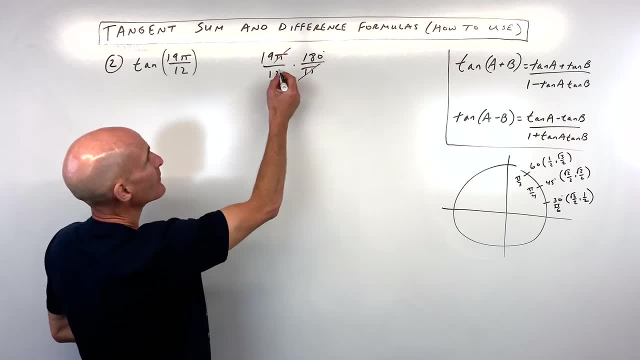 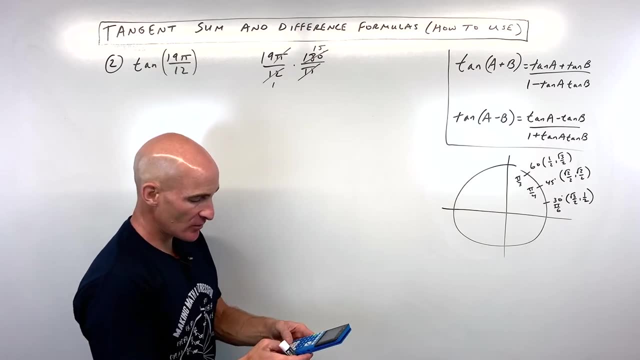 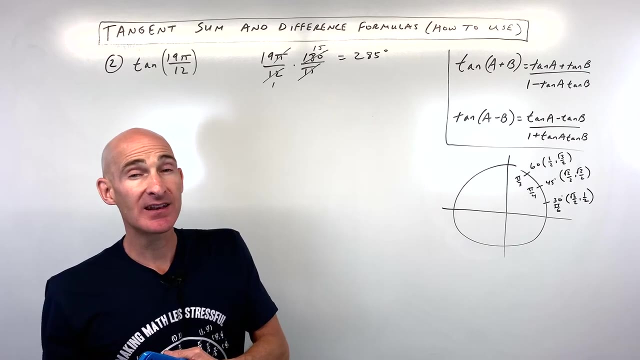 our conversion factor. Notice the pi's cancel. numerator and denominator 12 goes in here. once. 12 goes in here 15 times and 19 times 15, does anybody know what that is? 285.. So this is really 285 degrees. Now what two angles add. 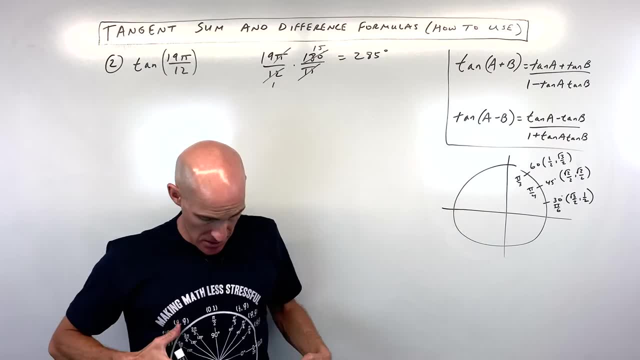 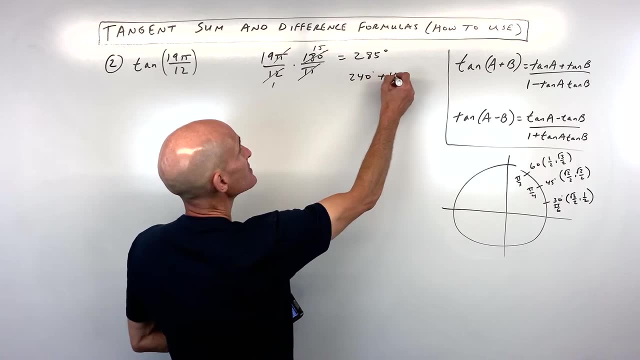 to 285, or subtract to 285 that you're familiar with on the unit circle here. Well, let's see How. about 240 plus 45? That adds up to 285.. But if we want to do this in radians, 45 is like pi. 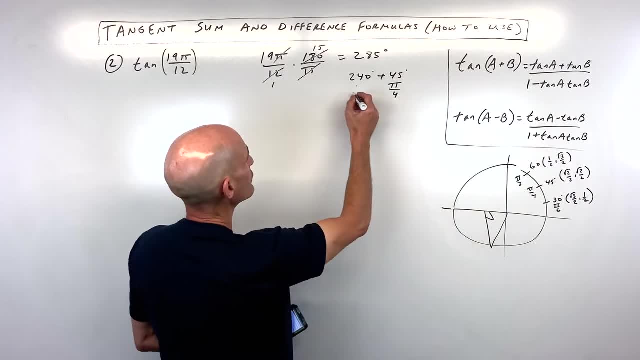 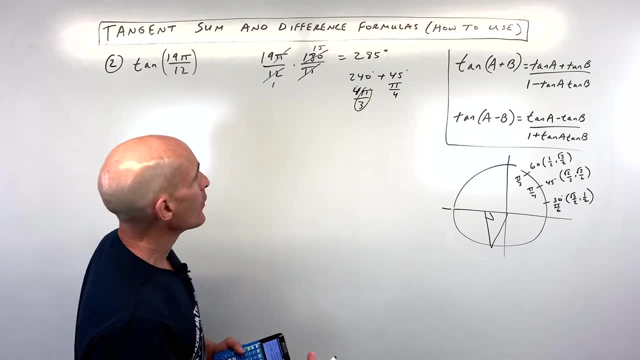 over 4, and 240 is how much 4 pi over 3.. There we go, See. one way to remember this is to see: pi over 3 is 60, and 60 times 4 is 240.. Okay, but basically. 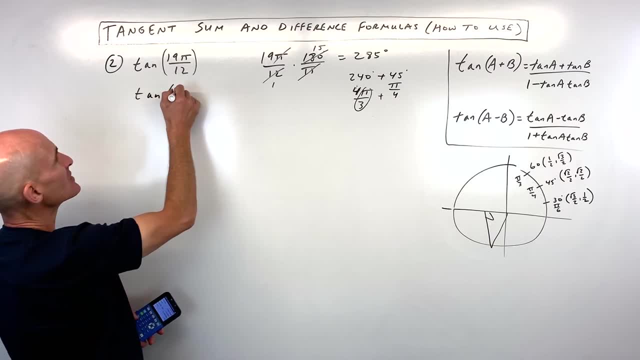 what we're going to do is we're going to add these two angles together. So let's rewrite that. So we have tangent of 4 pi over 3 plus pi over 4.. So this is our a value and this is our b value. So 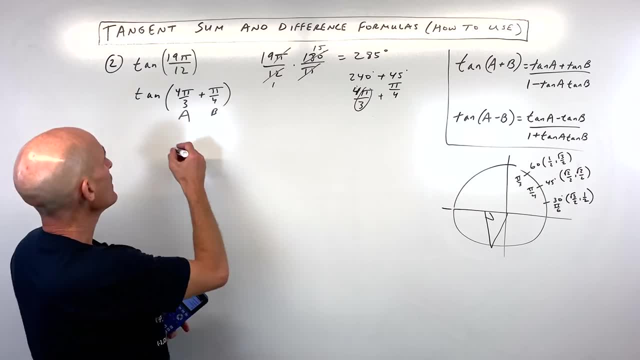 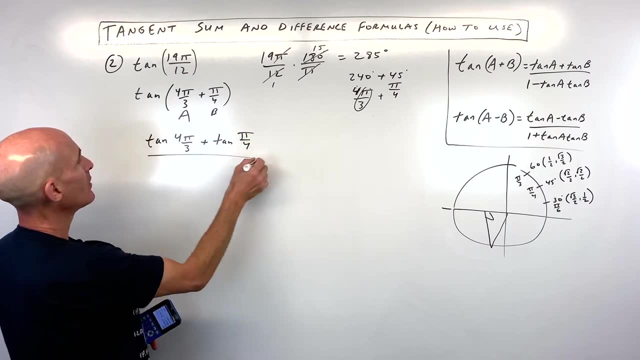 we're going to use our tangent sum formula here and let's expand it out. So we have tangent of 4 pi over 3 plus tangent of pi over 4, all over 1, minus tangent of 4 pi over 3.. 3 times the tangent of pi over 4.. Okay now, 4 pi over 3, we said was right here, right This. 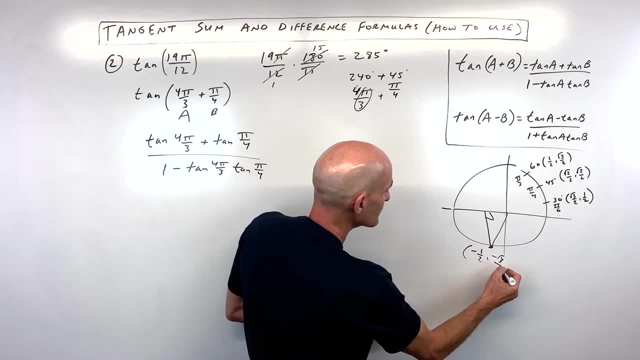 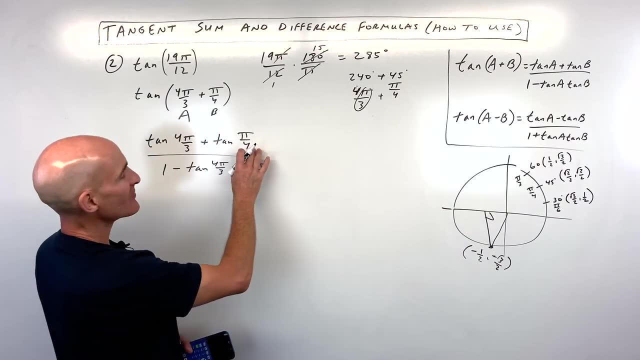 point is: at negative 1, half negative square root, 3 over 2.. Double check here, Okay, good. Yeah, exactly right. And if we do the tangent of pi over 4, that's right here. at this, 45, right here. 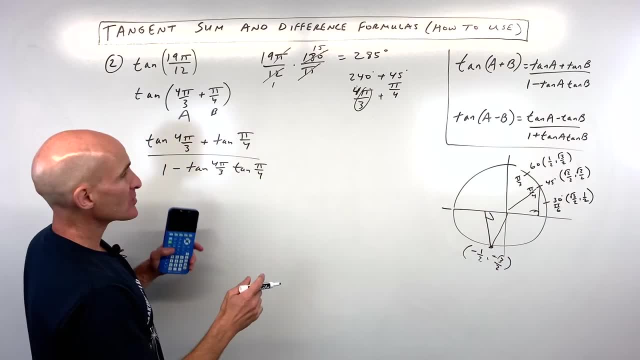 That's the root 2 over 2, root 2 over 2.. But remember, tangent is y over x, So we have negative root 3 over 2. divided by negative 1 half, That comes out to pi over 4.. So we have negative root 3 over 2. 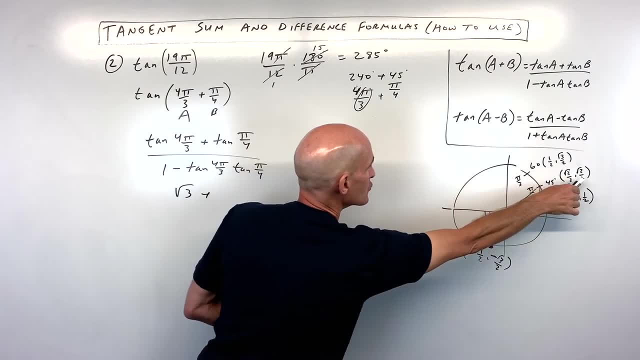 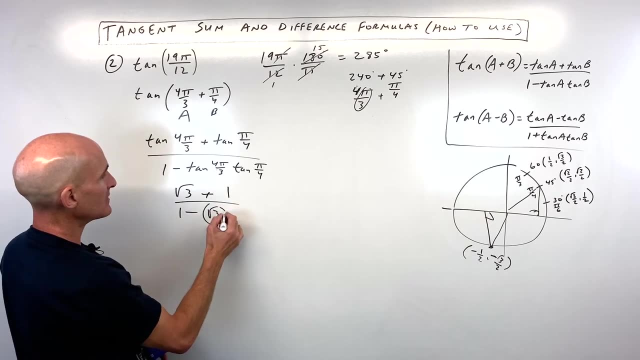 positive root 3.. Tangent of pi over 4,, that's root 2 over 2 divided by root 2 over 2.. That's 1. And 1 minus tangent of 4. pi over 3, we said that was root 3.. And tangent of pi over 4, we said that. 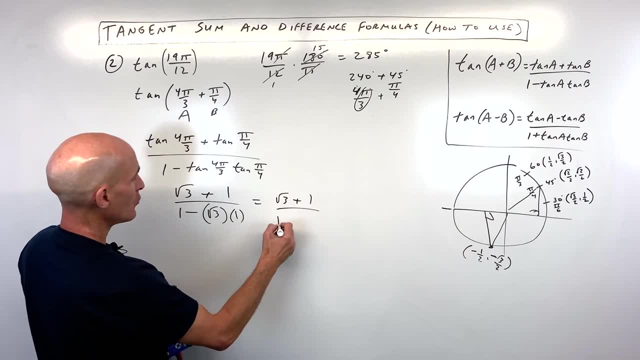 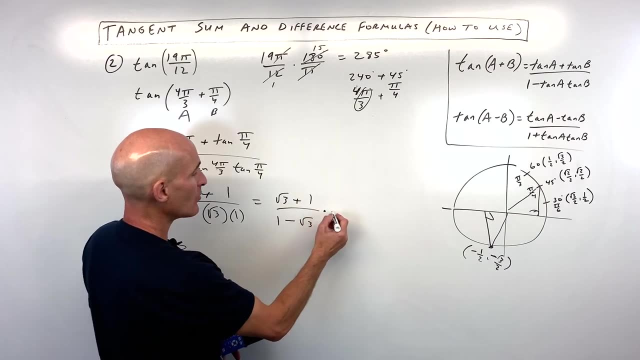 was 1.. So this comes out to root 3 plus 1 over 1, minus square root of 3.. Okay, so we could probably stop there. but to be more precise, more proper, I guess you could say: we want to rationalize We. 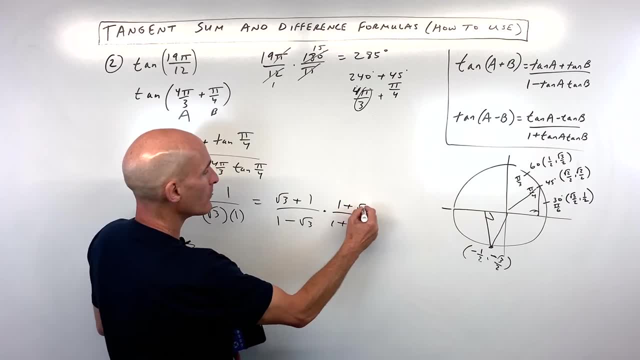 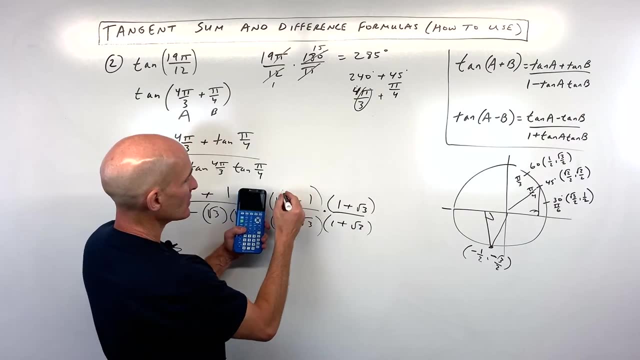 don't want that radical in the denominator, So we're going to multiply by 1 plus square root of 3.. That's the conjugate, And we're going to do some foiling, Okay so, or you can think about distributing twice. So root 3 times 1 is root 3.. 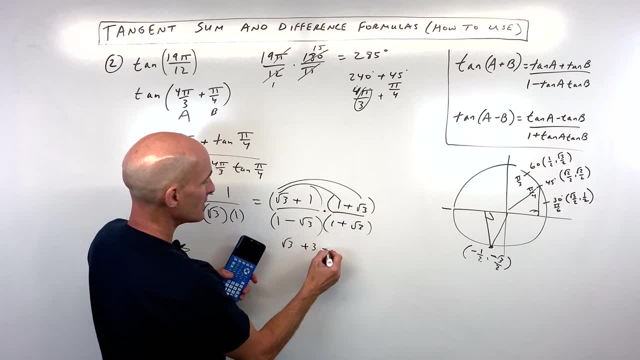 Root 3 times 3 is 3.. 1 times 1 is 1.. And 1 times root 3 is root 3.. In the denominator 1 times 1 is 1.. The inner and outer cancel And negative root. 3 times positive root 3 is negative 3.. So now, 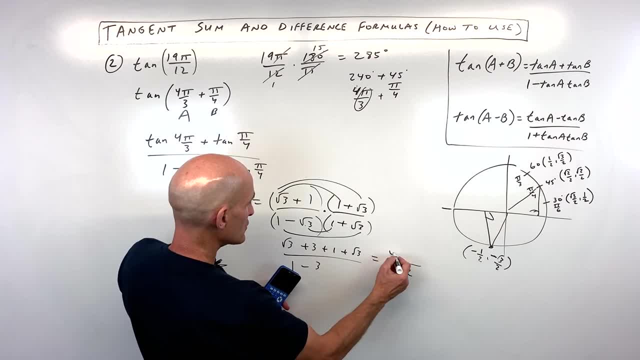 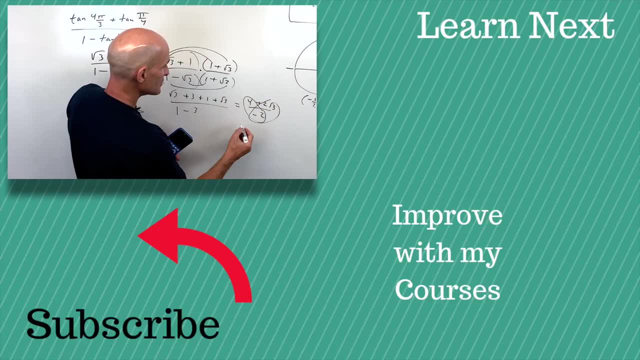 1 minus 3 is negative 2 in the denominator, 3 plus 1 is 4.. And root 3 plus root 3 is 2, square root of 3. And divide both of these guys in the numerator by negative 2.. So that comes out to negative 2.